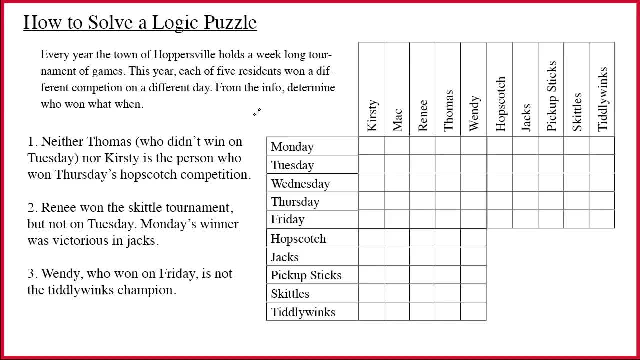 determine who won what when. So there were five days, five people, five games, and in logic puzzles you generally don't have to worry: hey, did somebody win two games? and things like that? No, it's usually a one-to-one-to-one correspondence. We're also given these. 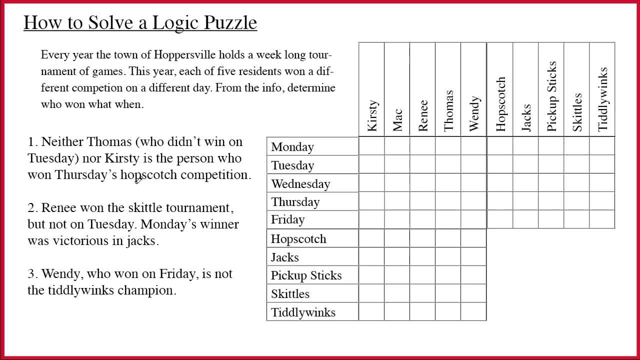 three sentences that provide some basic information. I like to think of these as the premises, and the first thing we want to do is extract the information from the premises and get it into the grid. So it says neither Thomas, who didn't win on. 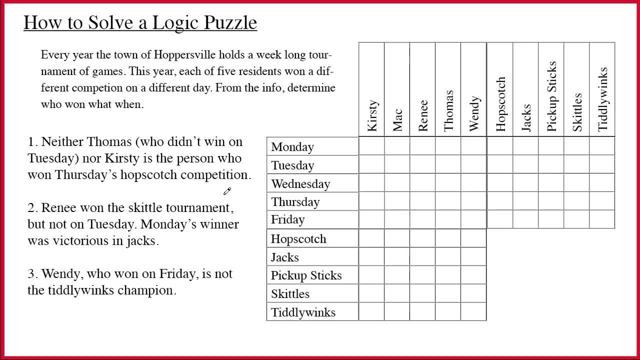 Tuesday, nor Kirstie is the person who won Thursday's hopscotch competition. Alright, well, that basically tells us that neither Thomas nor Kirstie won on Thursday, and let's use an X to denote a negative correlation. They didn't win on Thursday and they didn't win hopscotch, so some more X's. It also told us up here. 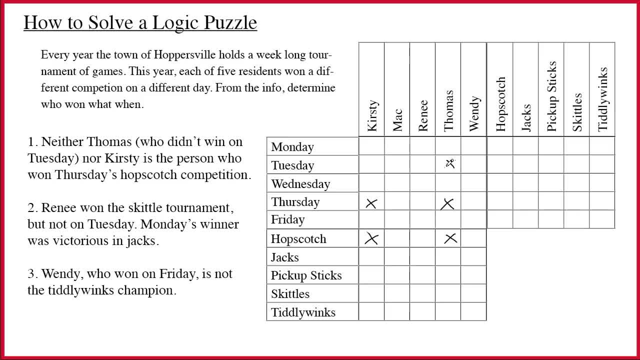 in parentheses that Thomas didn't win on Tuesday. and then notice there's one more really valuable piece of information. It says the person who won Thursday's hopscotch. Ah, so that means that hopscotch itself was on Thursday. Let's use a dot to denote a positive correlation. Now here's an example of the. 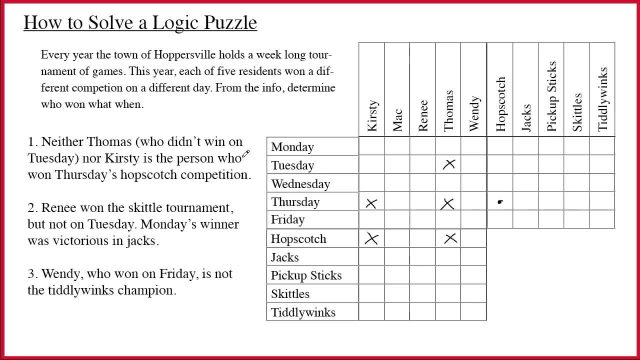 type of thing that I invite you to be thinking about as you're doing these puzzles and making connections with the sort of thing that you're doing. When I put in this dot, I can immediately put in all the rest of the X's in this column and in this row. You'll notice that the table here is composed of three. 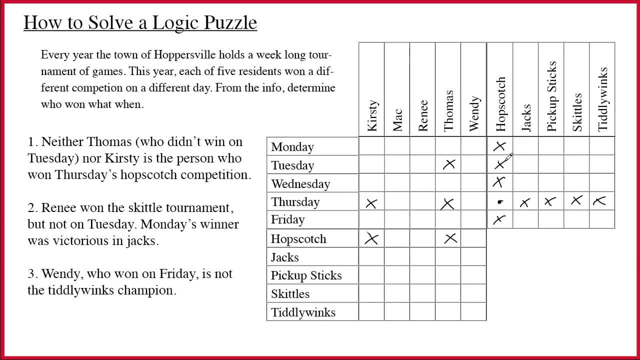 five by five grids, and as soon as you get in a dot, you get to put in all these X's as well. Here's the thinking that justifies this: If hopscotch is on Thursday, then it's not on Monday, and it's not on Tuesday and it's not on Wednesday. and 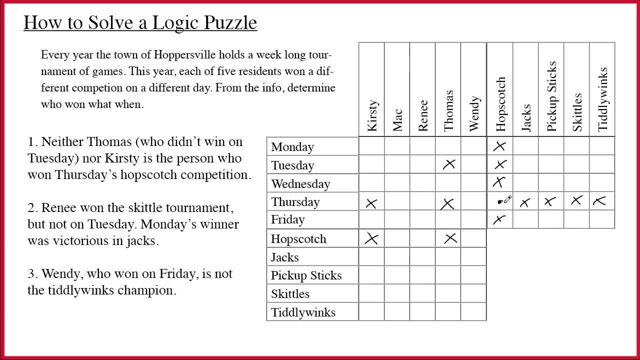 it's not on Friday, and if hopscotch is on Thursday, then neither Jack's nor pick-up sticks, nor skittles nor tiddlywinks was on Thursday. Notice that long sentence is just an extraordinary string of if-thens-ands-nots-and-or's. 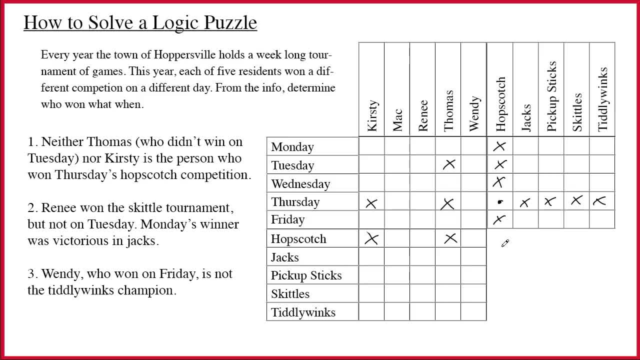 and you know, and yet we're sort of thinking these relations with incredible ease, All right. next sentence: Renee won the skittles tournament, but not on Tuesday. So Renee won skittles. There's another dot, and as soon as you put in a dot, go. 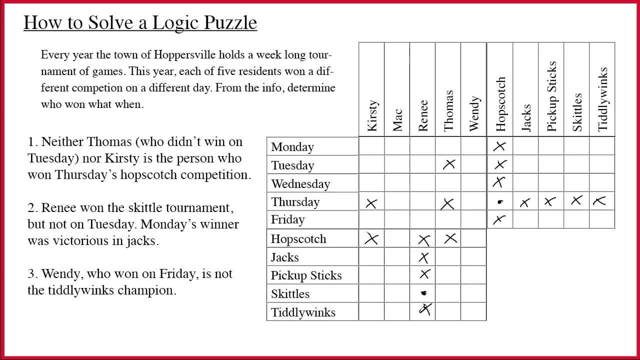 ahead and put in the relevant X's. She won skittles, but she didn't win it on Tuesday. So Renee did not win on Tuesday, but, moreover, that means that skittles couldn't have been on Tuesday, And so let's go to skittles and tiddlywinks. 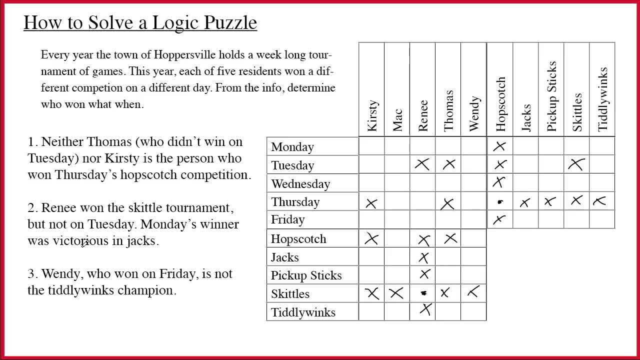 Tuesday and get another X. and then Monday's winner was Victorious and Jack's. So that means Monday and Jack's gets a dot right there, plus all the X's. Dots are good. Okay, third sentence: Wendy who won on Friday is not the tiddlywinks. 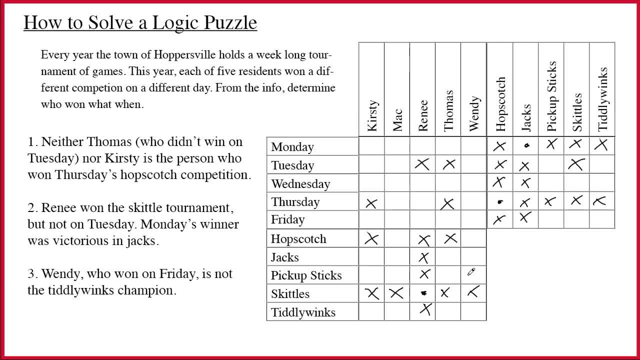 champion. All right, Wendy won on Friday a dot plus X's, but she is not a the tiddlywinks champion, And so that means we have to have an X here in tiddlywinks. And also, what does that tell us? That tiddlywinks couldn't have been. 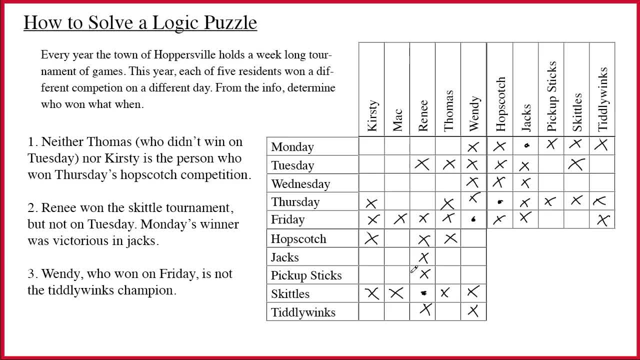 played on Friday. So another X. At this point we're done with the premises. We have extracted all the useful information and gotten it onto the grid, and now we can make progress just by comparing the three grids to each other. I should point out that in the bonus that I typically give at the end of the 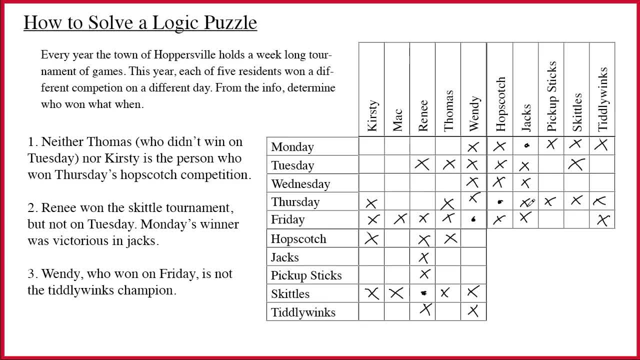 semester. once you've extracted the information from the premises, you make some progress, and then it's a good idea to go back to the premises, and sometimes one or two of those premises will actually provide you additional information later on. So this is an especially easy sample puzzle. But after 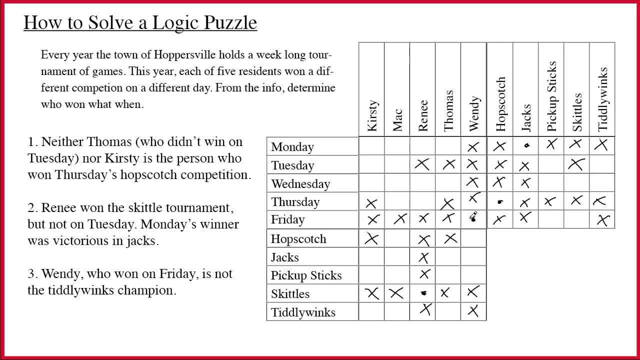 you've extracted all the information. a great way to make progress is to focus on the dots. So notice, this dot tells us that Wendy won on Friday. Well, what games could have been played on Friday? And notice, the answers are: pick up sticks and skittles. 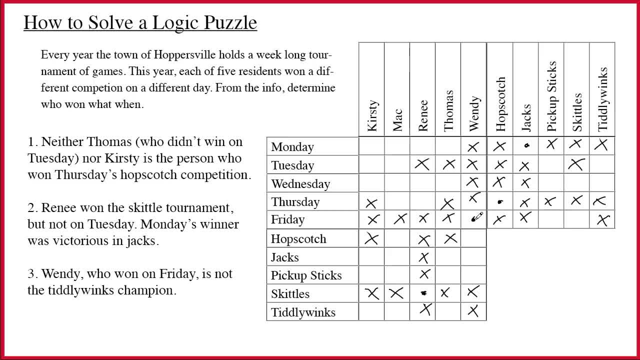 So that means that Wendy had to win either pick up sticks or skittles. But if we go down here, it tells us that she didn't win skittles. Therefore, the only thing she could have won would be pick up sticks. So we'll put in the dot plus. 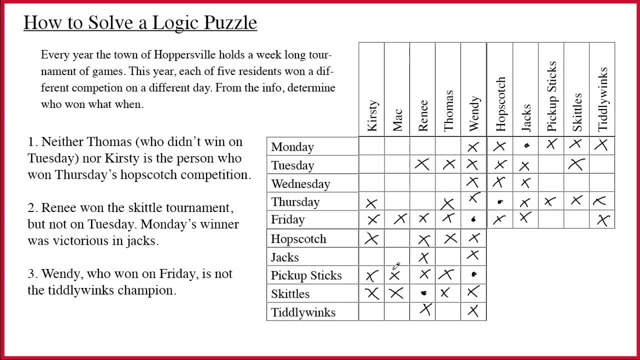 the X's Notice what we actually just did. We said Wendy had to win either pick up sticks or skittles. In symbols that would be pick up sticks, wedge skittles. But then we said she couldn't win skittles, so that's not skittles. Therefore she had to win pick up sticks. 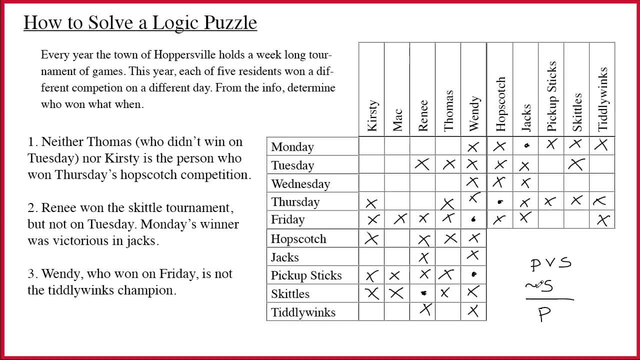 We actually just did disjunctive argument, but we did it in a really intuitive and simple way. So if you make a little bit of effort to sort of think about consciously what you're doing in your head as you're doing the logic puzzle, that's really what I have. 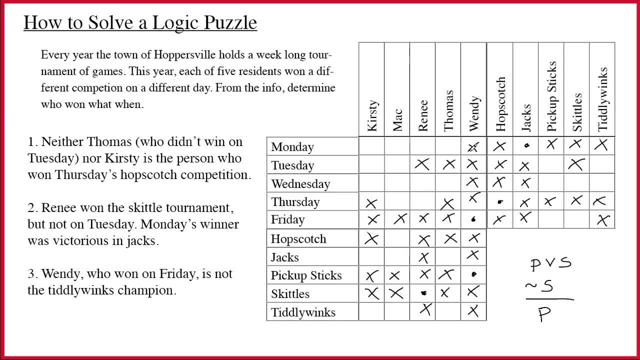 in mind. So notice, we said that Wendy won pick up sticks. We know that pick up sticks that Wendy won on Friday, that means that pick up sticks itself had to be played on Friday. So dot plus X's. And now notice what just happened in this. 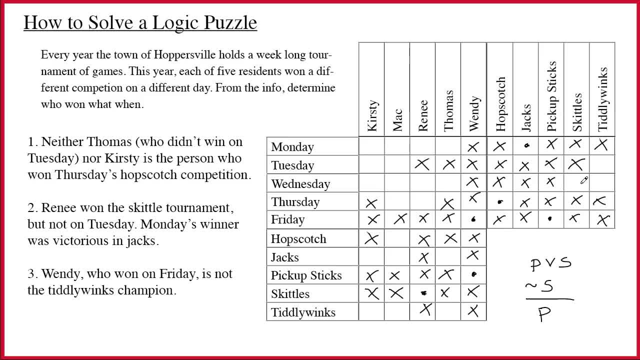 five-by-five grid. In the skittles column, the only day that's left is Wednesday, So that had to be the day it was played. Tiddlywinks therefore had to be played on Tuesday. We have finished this five-by-five grid. Notice: there's one dot per column and there's 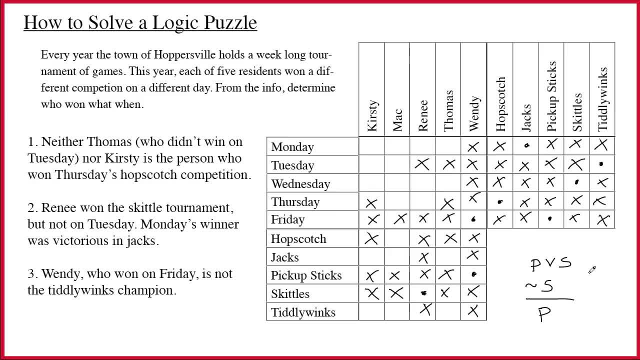 one dot per row, and that's always the way that it should be. Alright. so all of that happened because we started with a particular dot. Sometimes the dots are this helpful, sometimes they're not. Sometimes, if you, if the dots aren't helping you, it's great to start where you have just a 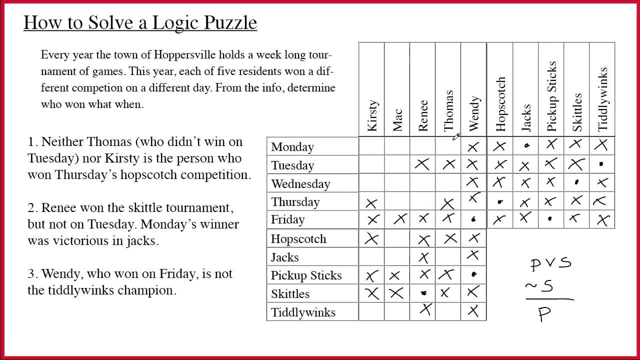 couple openings. So notice, we know that Thomas won on either Monday or Wednesday. Well, that means that he had to win either Jacks or Skittles, because that's the games that was played on those. those are the games that were played on Monday and Wednesday. So let's take a look- Jacks or Skittles- And we come down here and we